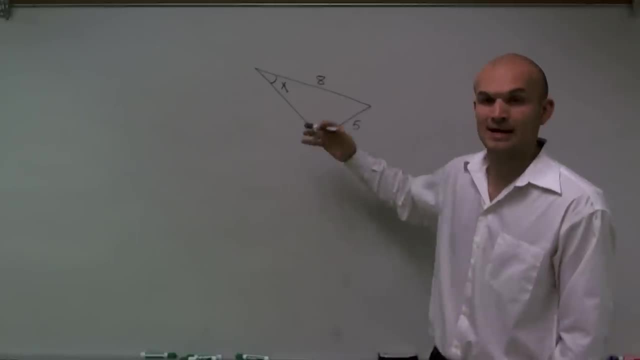 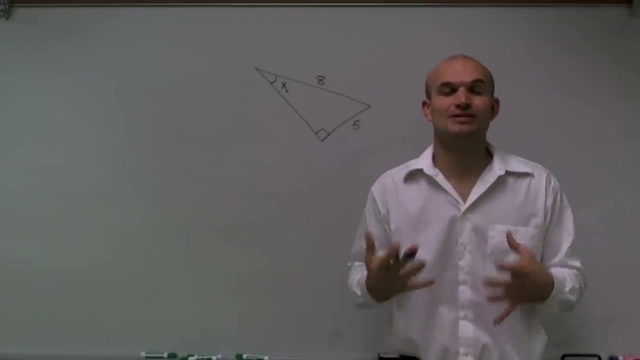 this little square at this angle, And what that represents is I have a right angle And when I have a right angle, I have a right triangle And when we have a right triangle. it's very important for us to understand that, because there's a lot of things we can do when we have a right triangle. 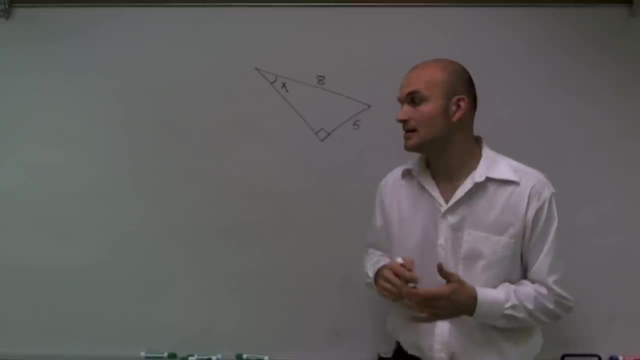 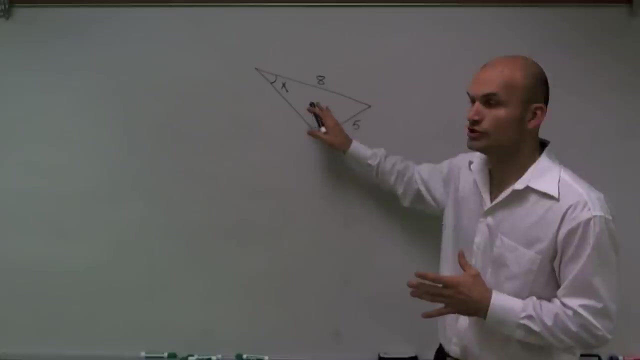 One is: we can apply the Pythagorean theorem when we're dealing with side lengths, But here we need to find a missing angle. So when we're using our missing angles, it's really helpful for us to use three trigonometric functions, And I want to kind of go through this and explain your. 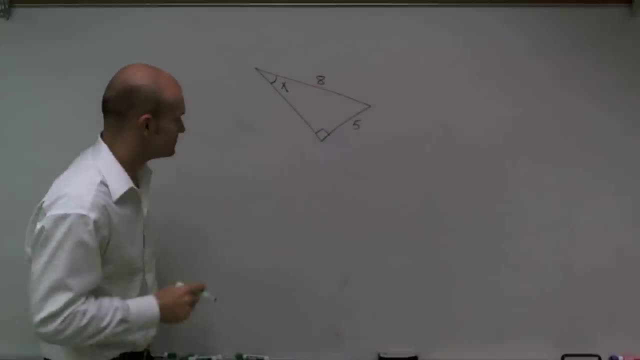 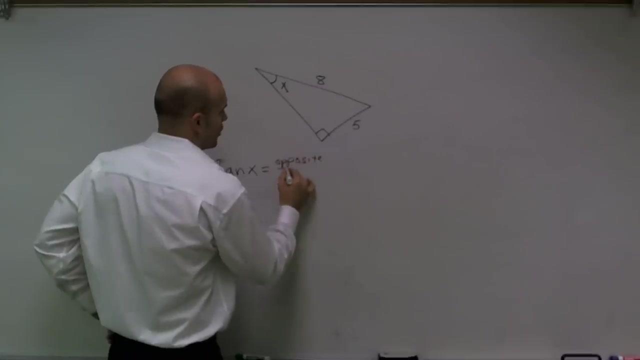 trigonometric functions to help you understand them. So, when we have a trigonometric function, the first one I want to talk about is our tangent. So a tangent of an angle x is equal to the ratio of the opposite side over the adjacent side. All right, now, that's one ratio, or one trigonometric ratio. The next one: 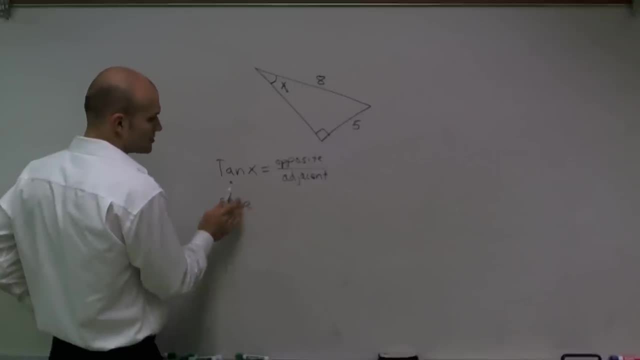 is your sine function And usually we just abbreviate your sine as S-I-N. So sine of x is equal to the ratio of the opposite side length over your hypotenuse And the cosine of x is equal to your adjacent over your hypotenuse. Now I just started abbreviating. 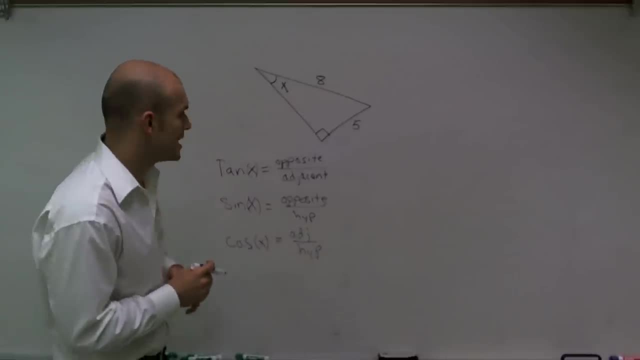 these, just so you guys get used to this. but to your adjacent over your hypotenuse. Now you might ask me, well, where I kind of remember hypotenuse from doing the Pythagorean theorem. but where did your adjacent and your opposite come from? Well, if I'm going to look at my angle x right here, 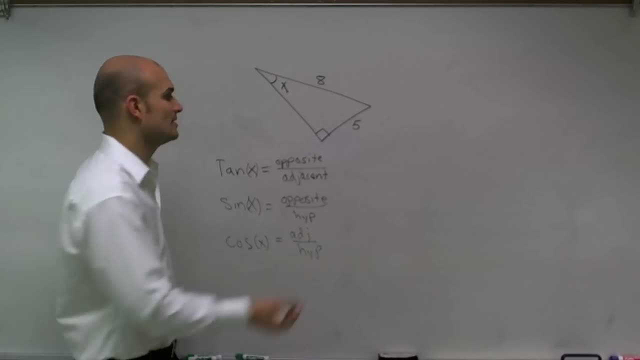 we know that the hypotenuse is always going to be the longest length, right? Well, another way to remember that is, your hypotenuse is always directly across from your 90-year angle, So it doesn't matter what I do to. 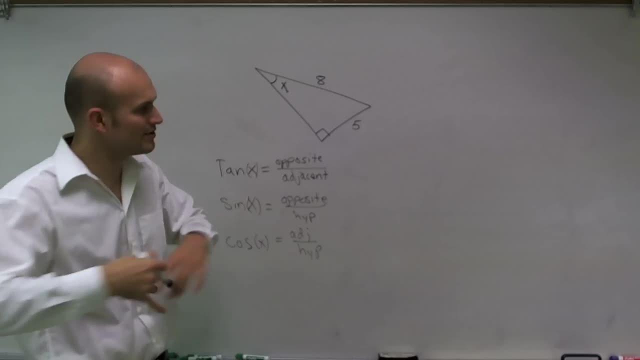 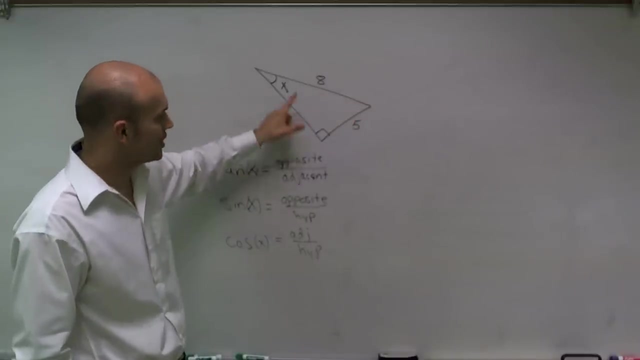 my triangle. I can flip it, reflect it, do anything I want to it, wrinkle up, strangle it, throw it back up there. My hypotenuse is always going to be my longest leg, or longest length of my triangle, And it's also going to be directly across from my 90-year angle. Now, the opposite. 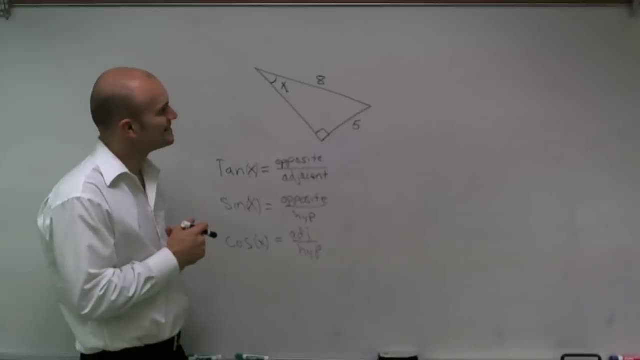 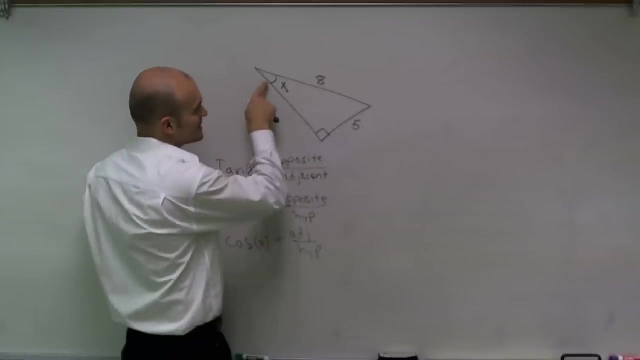 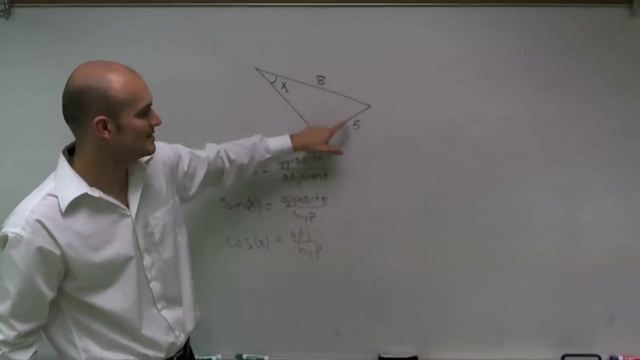 excuse me, the opposite and adjacent angle. let's come in where the opposite is directly across from your angle and your adjacent connects your angle to your 90-year angle. So what we can see is: I have my hypotenuse is eight, and then 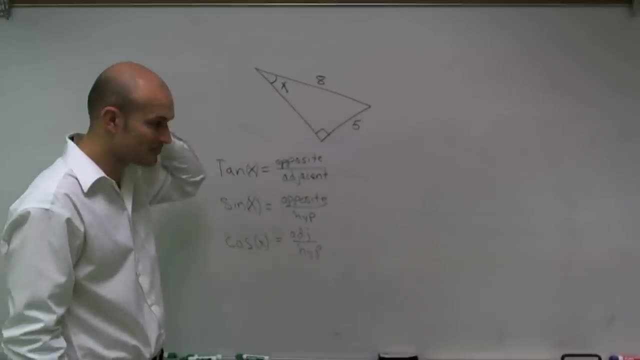 what I have is my opposite side because it's directly across from my angle x. So I need to look at which tan function talks deals with my opposite and my hypotenuse, And what I look at is I can see the sine function deals with opposite over hypotenuse. So therefore I'm just going to kind of forget. 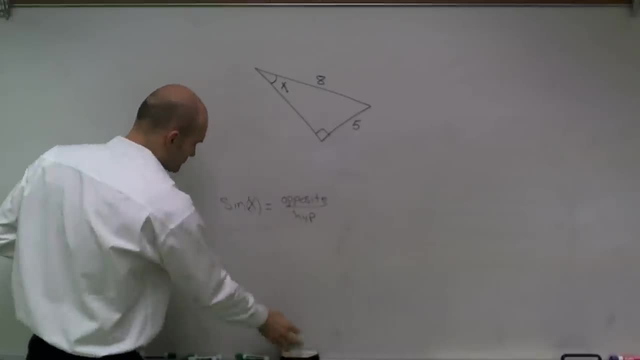 about the tangent and the cotangent. So now I have: sine x equals the ratio of the opposite side over the hypotenuse side. So now what I need to do is say: well I know, the opposite side is equal to 5.. And 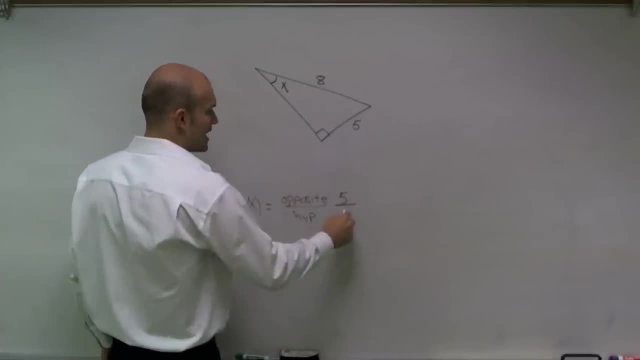 the hypotenuse- I'm sorry, the opposite side- is equal to 5, and the hypotenuse is equal to 8.. So I have: sine of x is equal to 5 divided by 8.. Well, let's go and see if we can get a decimal approximation. 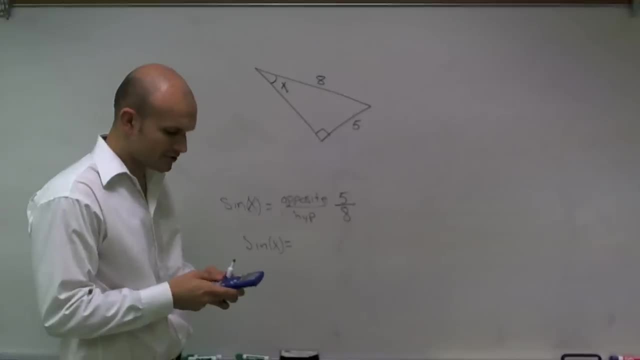 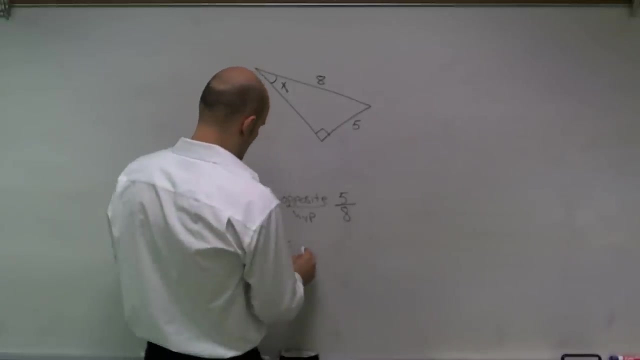 for that, just to kind of show us what we're going to do. So I take 5 divided by 8, and I get 0.625.. So what that says now is we have the sine of our angle x equals 0.625.. 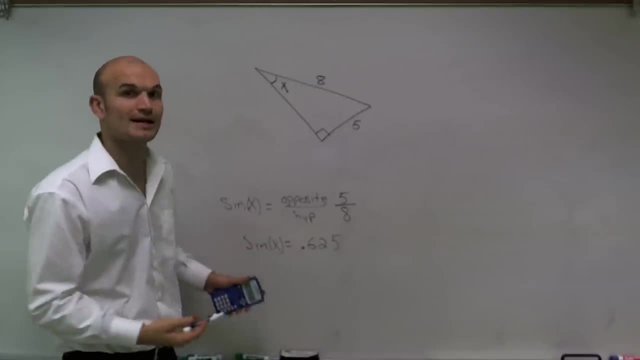 But we want to find out what is the value of x. So what I need to do is I need to undo my sine function, And what we call this is to undo your sine function. we need to look at what we call the inverse of the function. 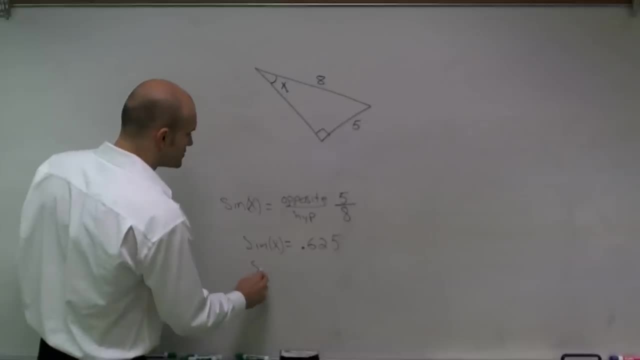 So what we're going to do is we're going to plug in To undo sine. we need to use sine inverse. So if we're going to undo sine, we want to undo the sine inverse to our value, of our function, which is 0.625.. 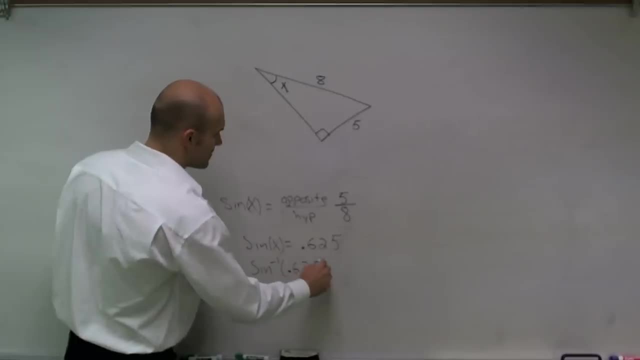 So I'm going to say inverse sine of 0.625.. And what that's going to give me is that now is going to give me the value of my x, which is my missing angle. So what I'll do is I'll take a graphing or a scientific